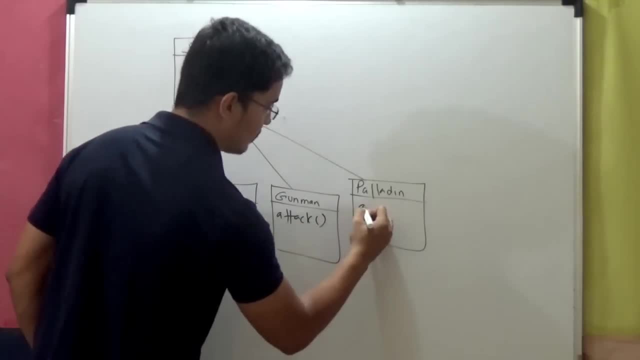 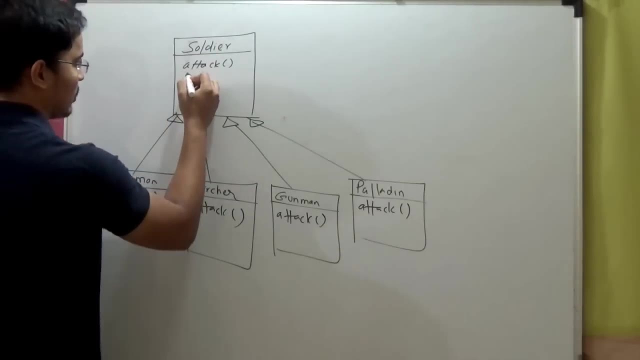 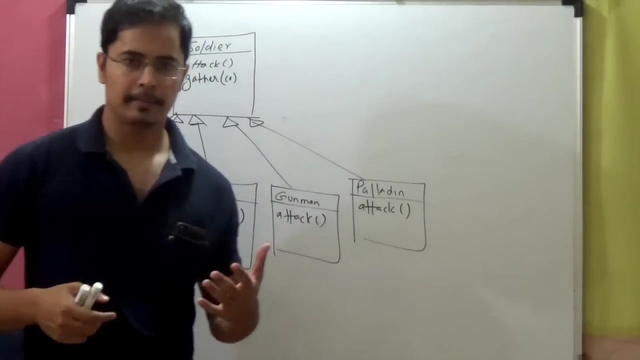 And gunmen will use guns. So that's why this method is implemented differently in different specific type of classes. There's some common method in the Soldier abstract class, that is gather with some coordinates. Imagine you are a soldier, You are a developer who is developing this game. You are in the development team. 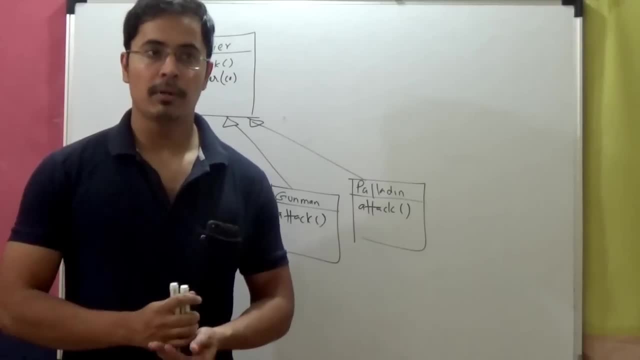 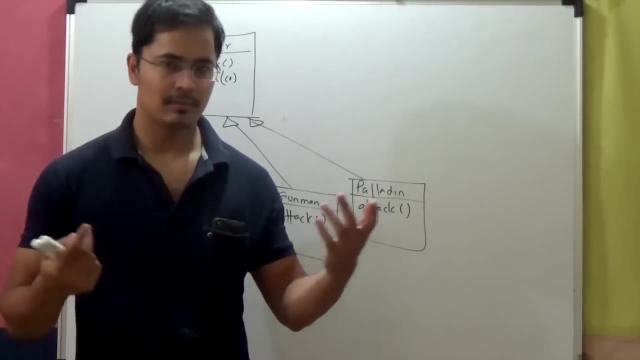 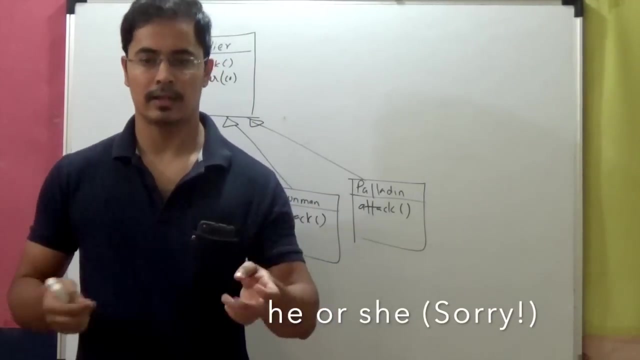 So your immediate boss has asked you to implement a functionality of refill. Refill the weapons So in the older versions of the game, as long as the soldier is alive, he can keep attacking with his weapon. But you want to simulate the refill behavior that. 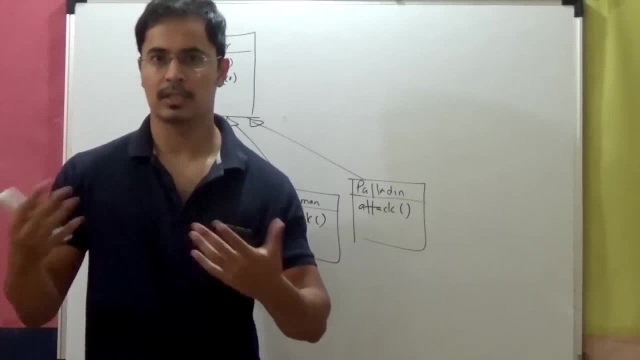 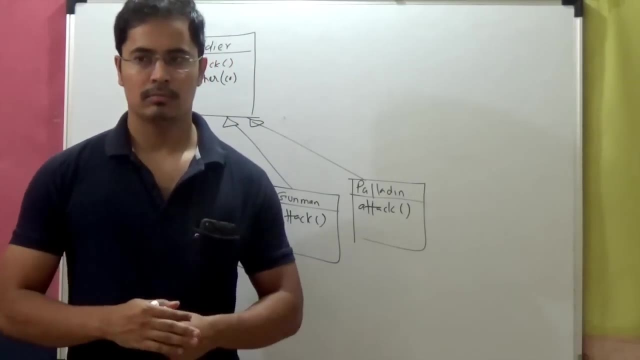 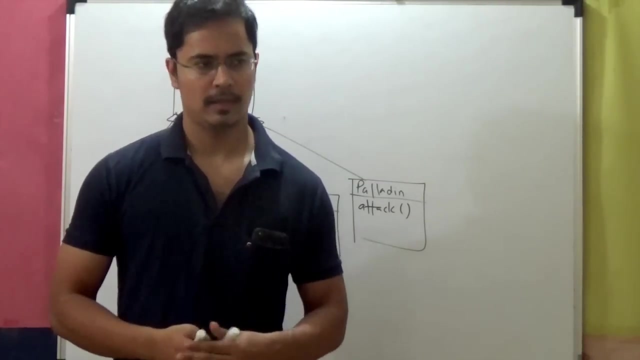 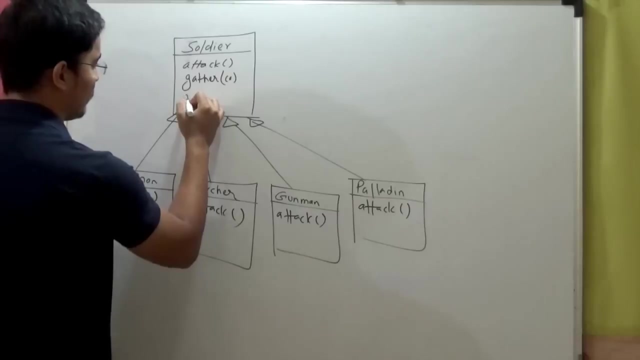 he will run out of ammunition And after a specific interval the soldier will have to refill the weapon. So there's a quick demo to the upper hierarchy of bosses and you need to quickly implement this solution of refilling. So as a developer, my first instinct will be: I'll put a refill. 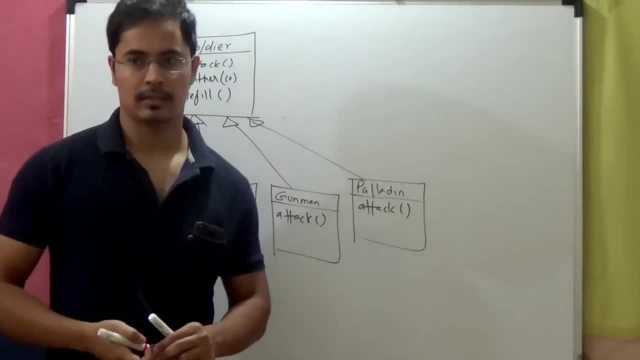 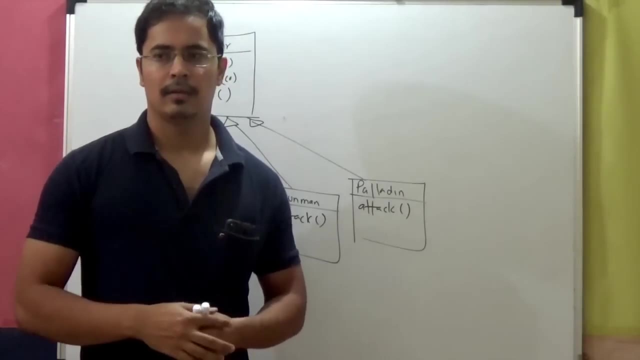 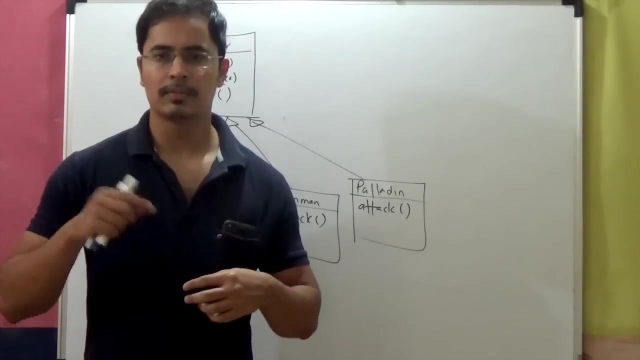 method. here in the base abstract class of soldier, This refill method will be something like: after a specific interval of time, Let's say ten seconds or something, The soldier will stop fighting and will spend some time in refilling the weapon and then continue fighting, right? So because you kept this concrete, 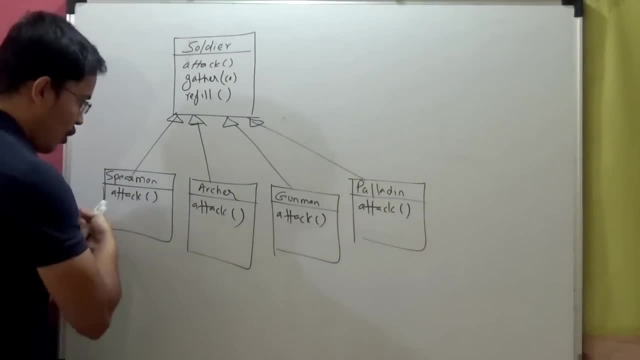 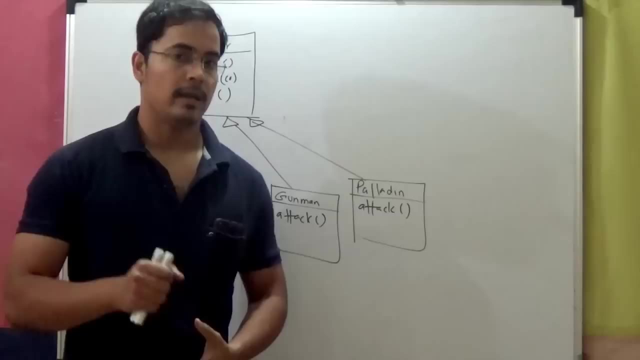 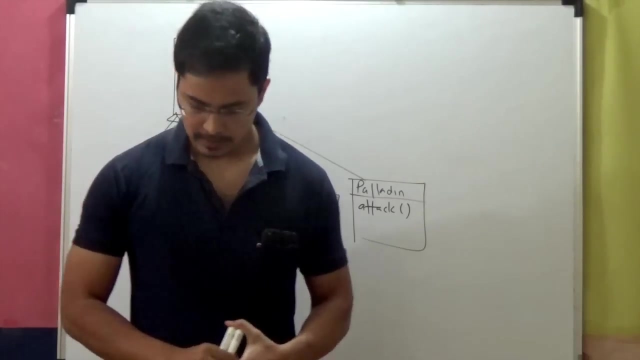 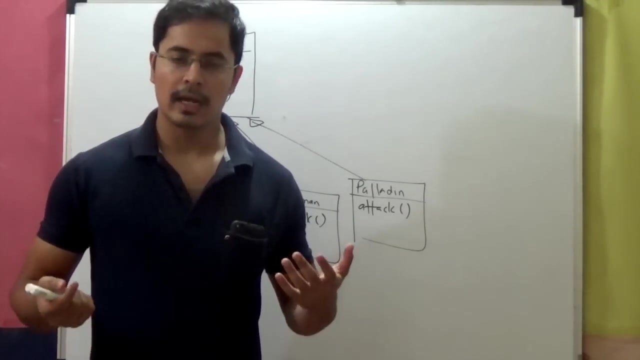 method in your soldier abstract class, all these specific types of soldiers will automatically get that refill behavior right Now the demo happened and guess what? It wasn't that good. What happened? so your immediate boss has come back to you with the feedback: that man, what the heck you did you. 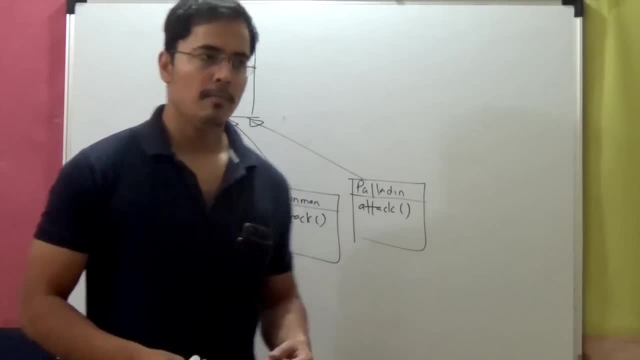 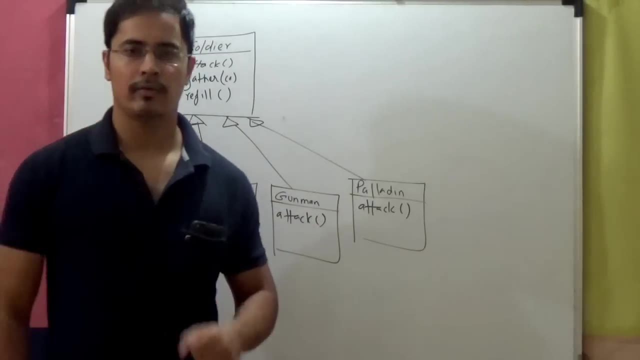 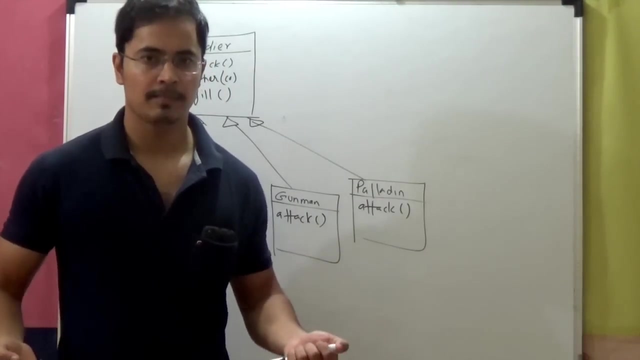 should have some common sense. i said why? because why will spearmen or paladin need to refill their weapons? spearmen have spear, paladins have swords. they don't need to refill their swords or spears. so because i implemented it, like you know, after certain period of time, gunman and archer will just 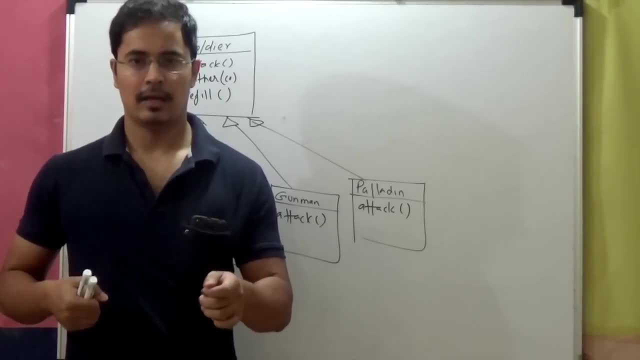 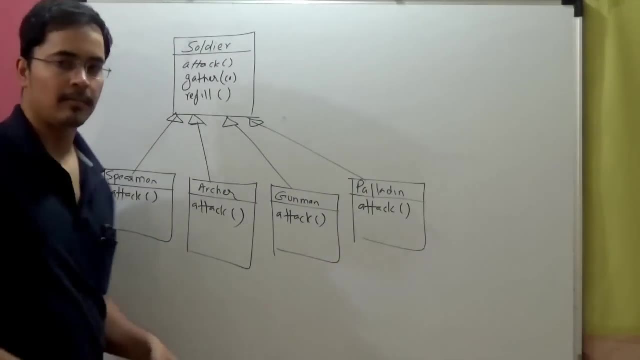 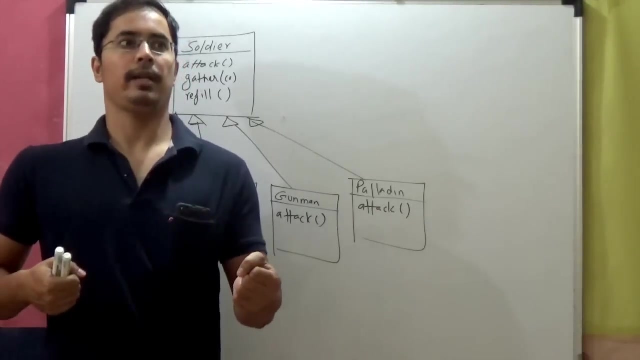 stay stationary for, let's say, few seconds, uh, indicating that they are refilling, and then again they will start fighting. so, unfortunately, what happened is that my spearman was also fighting and because it also got this refill behavior after that specific time, he stopped fighting for certain period of time and again started fighting. 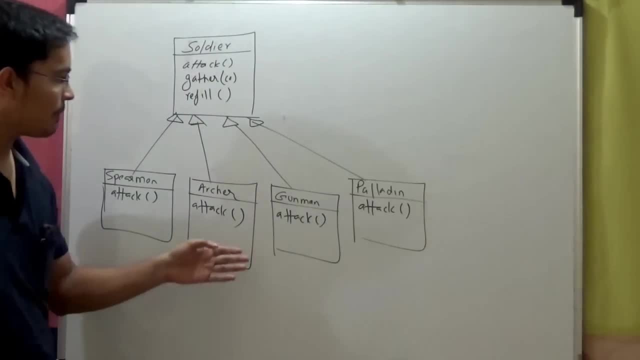 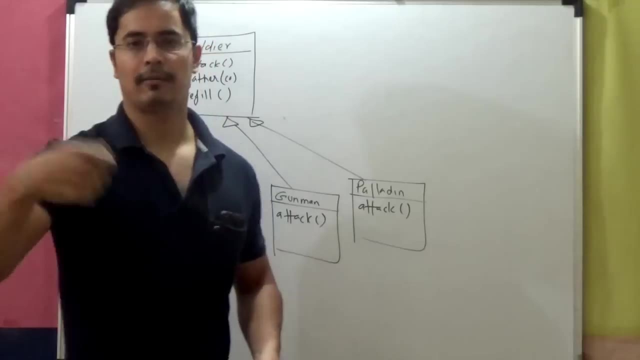 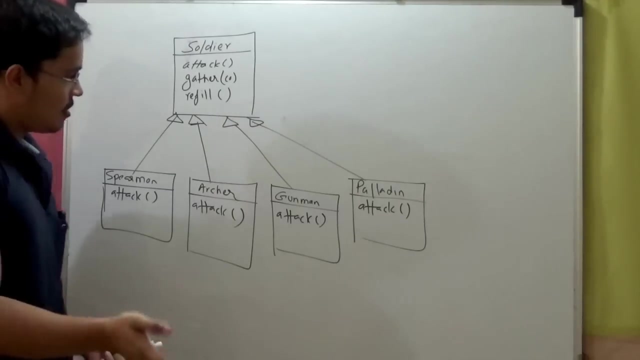 so it was really funny. and same thing happened with paladins. they were really fighting a lot and statue and then again start fighting. so yeah, not not a good site in the demo right, so that's a problem. so i was stupid. maybe i was hard pressed by the demo deadline, so i should. 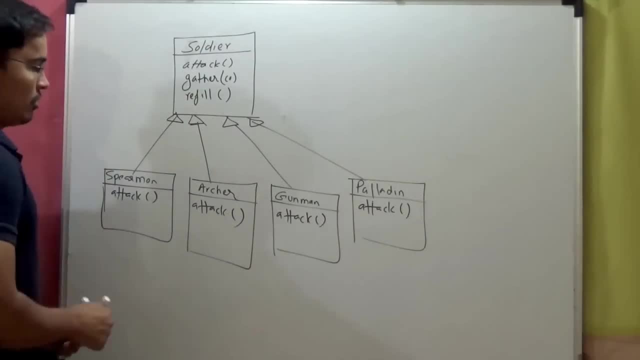 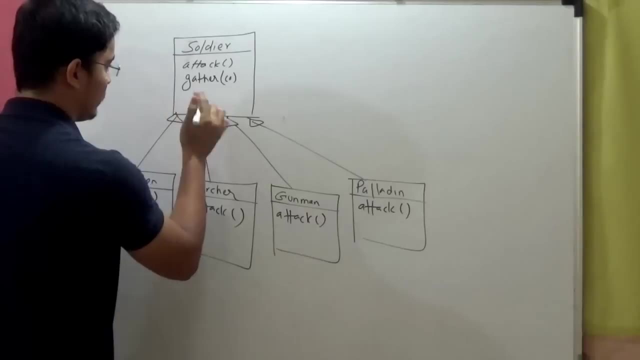 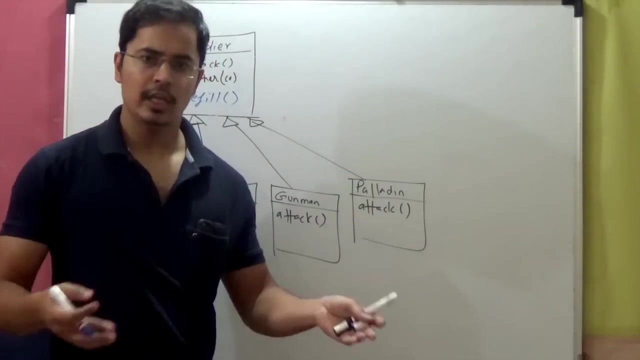 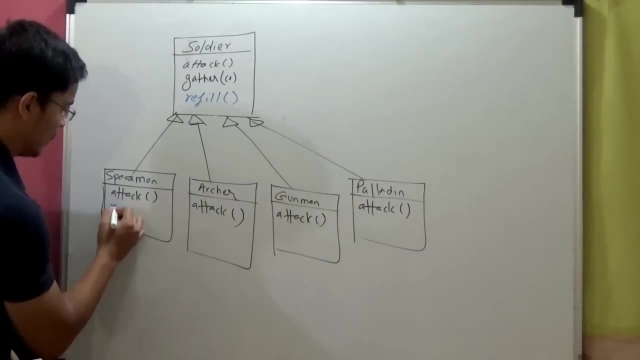 not have put it here right. so then i think, okay, i can, i can make this abstract right, so i can say italic. and this will be like attack: it will be individually implemented by each, uh, specific type of soldier. those who need not need to refill will do nothing, like spearman refill method will have no code, like nothing right, just blank. 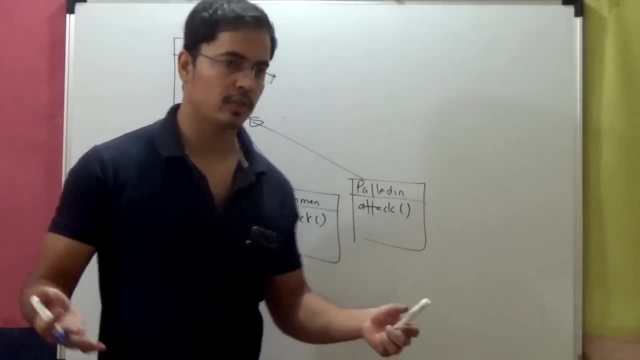 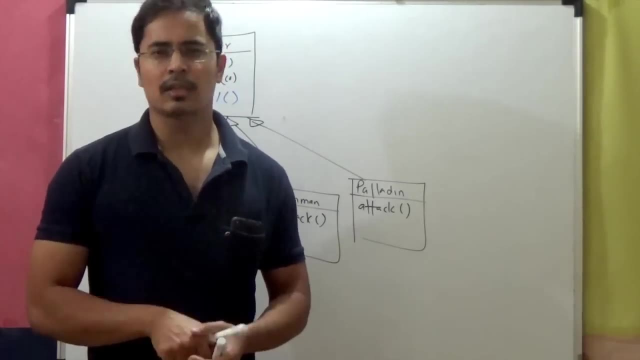 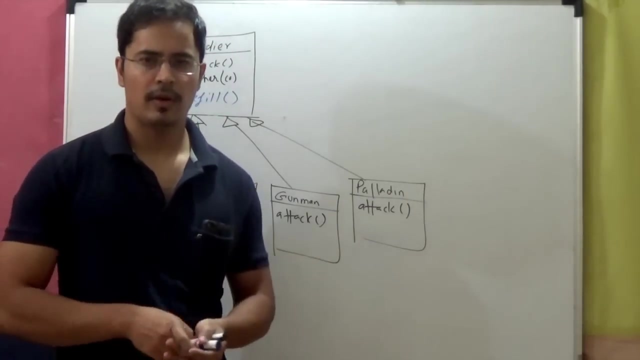 and archer and gunman will have some implementation for this refill method. right, that is, that is what i thought. but then is this a good approach? is this a good idea? i mean, if i think just right now, if i don't think much, maybe it is. but imagine tomorrow new requirement comes. 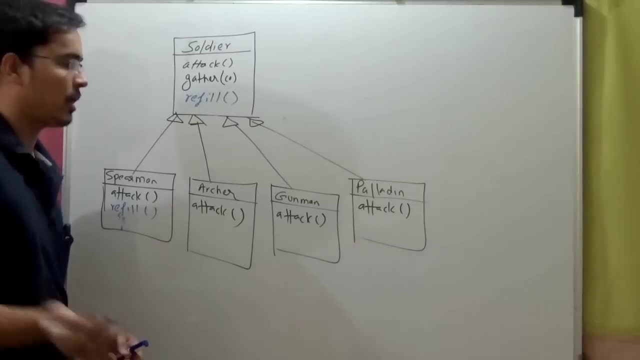 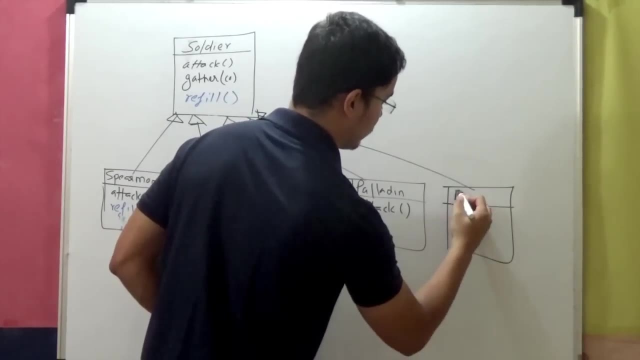 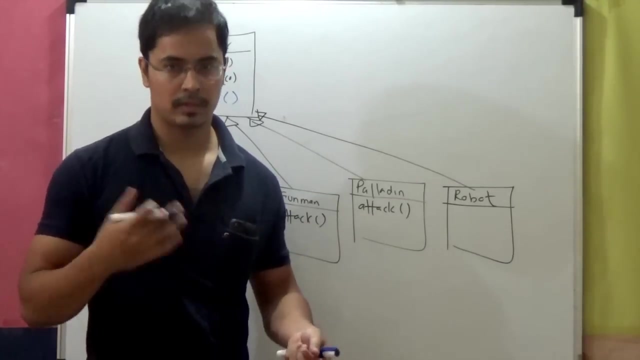 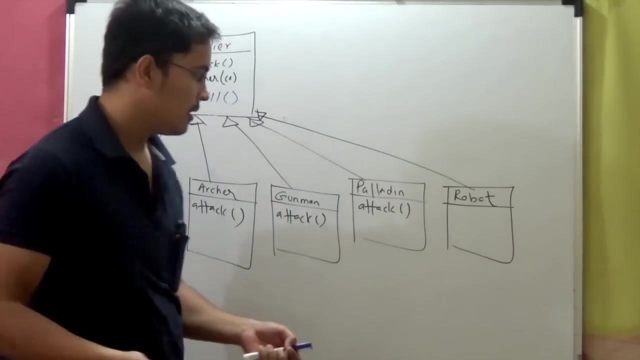 now that company is saying that we'll add one more type of soldier, which will be a robot. right, robot will need to not only refill the weapon after some time, but they also want robot to have repair method, repair behavior, because you don't want just robot to get killed straight away. it. 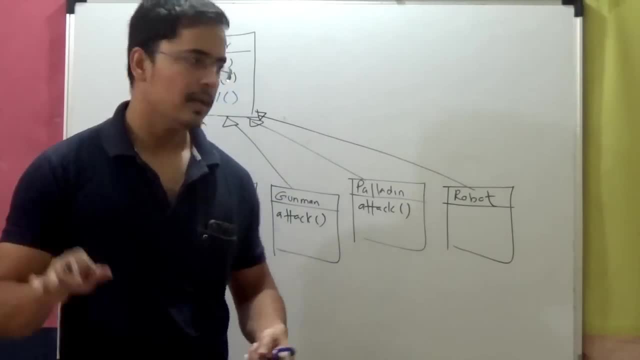 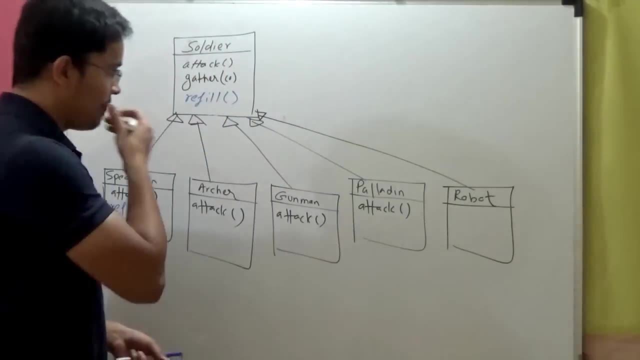 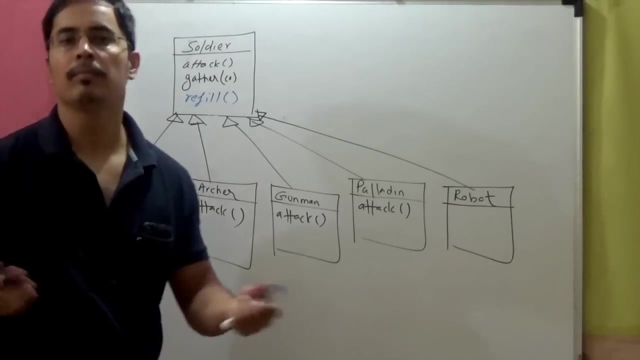 might get damaged after certain attack, certain period of attack, and then you might want to repair the robot. you might want to give that option to repair the robot rather than just killing that robot. okay, so i was thinking that refill i will make abstract and some classes will provide no implementation, like blank implementation, and some classes will implement. 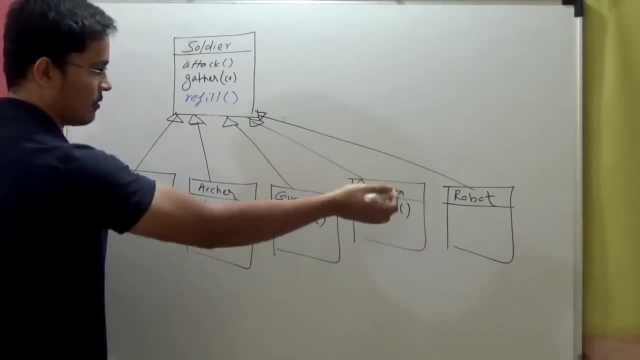 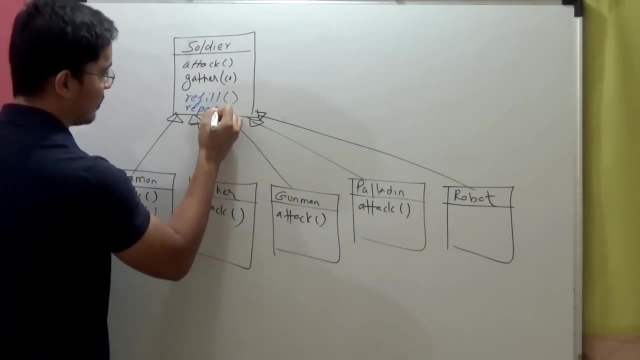 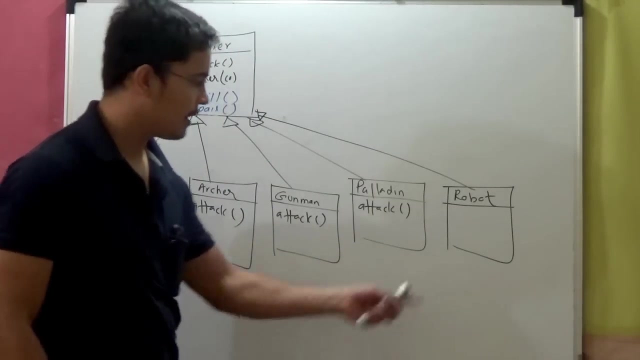 it now. i have another problem now to keep this one more method called as repair. because of this new type i will make it abstract. then again, only robot is requiring this repair behavior. so repair will have some concrete implementation in robot. everybody else will say no behavior. or let's say: 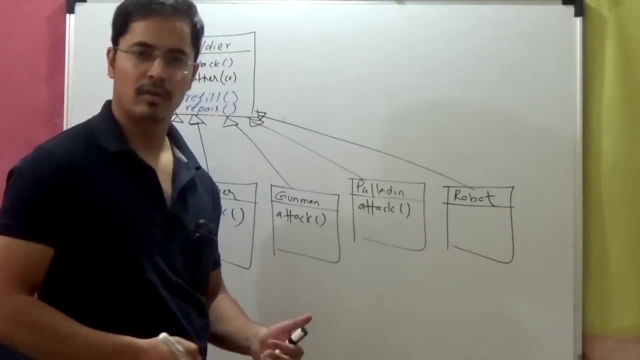 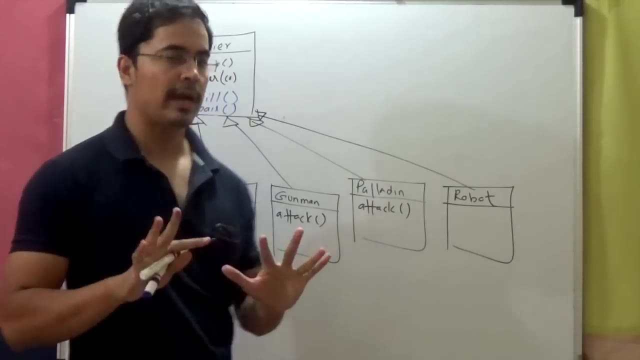 we're implementing that repair abstract method doesn't sound good, right? i mean, these guys don't need any repair functionality, so not a good approach. so i thought inheritance was a good idea in this case. you know, they're all soldiers basically for code reuse, but this is more like a 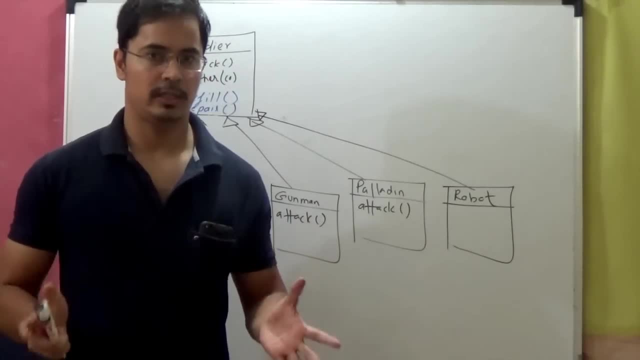 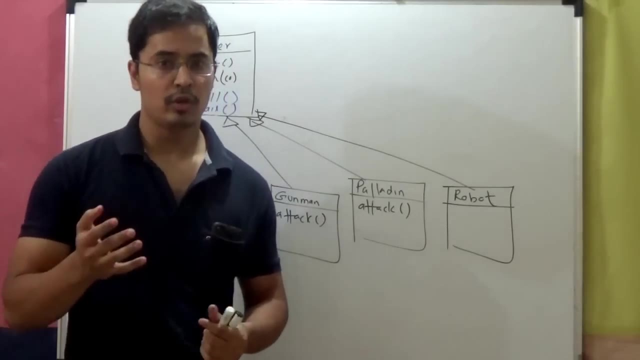 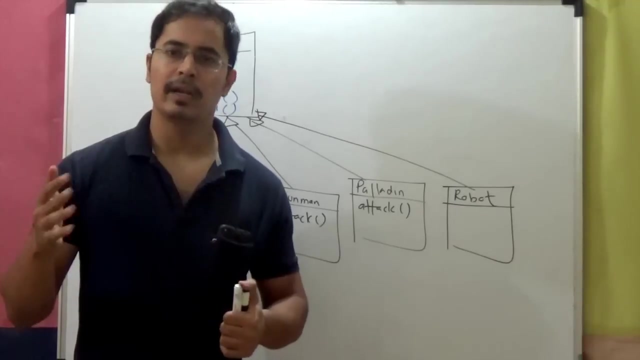 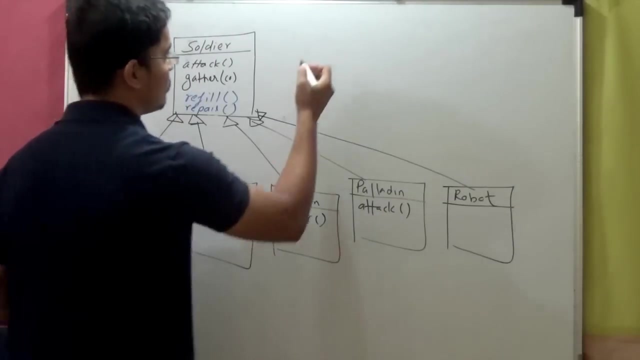 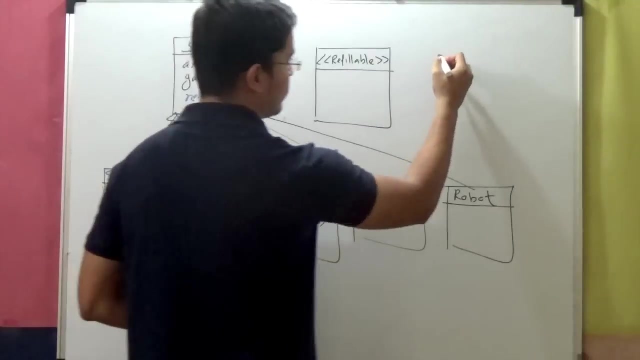 code replication. so inheritance is not really working much here, right? okay, not inheritance, then what? maybe we could use interface? yeah, i mean, interfaces are like, not that binding, they are much more loosely coupled, right? so what i will do is i'll write two interfaces, refillable, right, and one repairable. i know the symbol of interface. 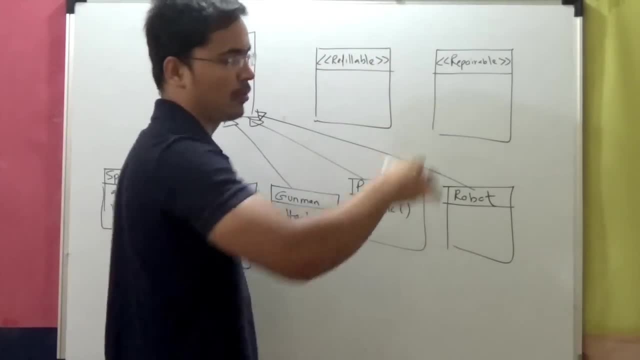 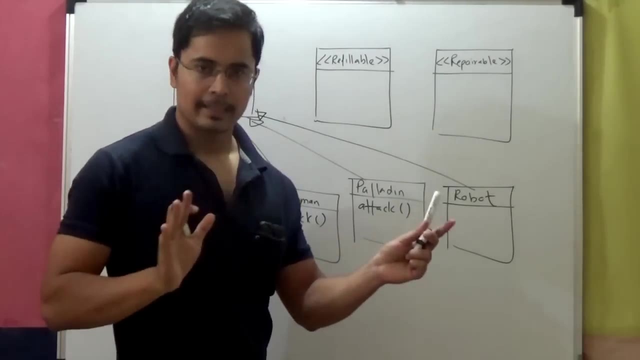 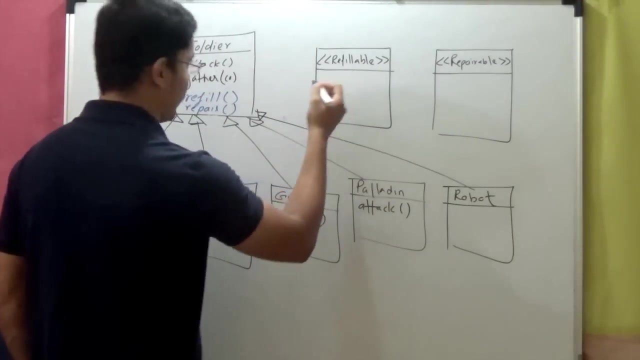 is a bit a bit different. like you write interface and then below that you write: but imagine, so we have learned class diagram. right, you know the exact notation. i'm just a bit uh, i don't have enough space so i'll use that. okay, so do you know the correct notation? cool, so they will have refillable interface, will have some. 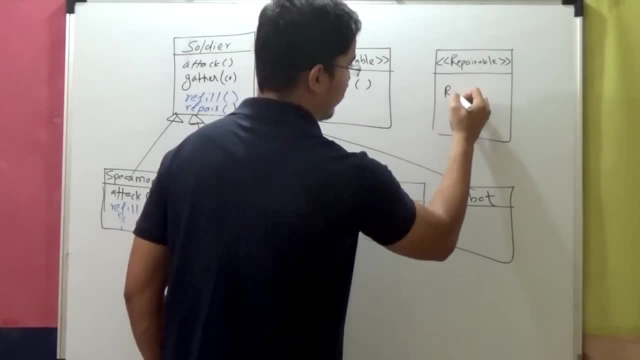 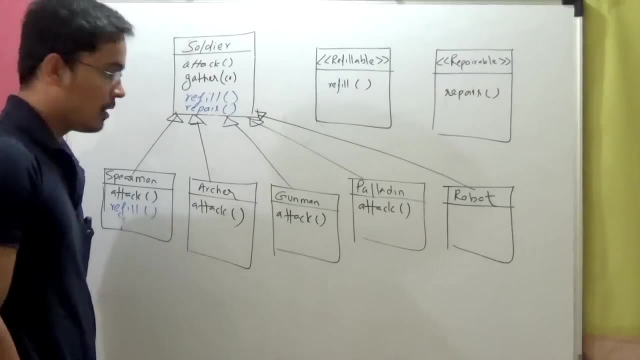 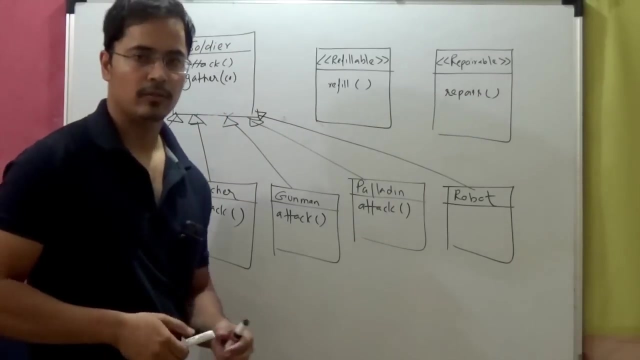 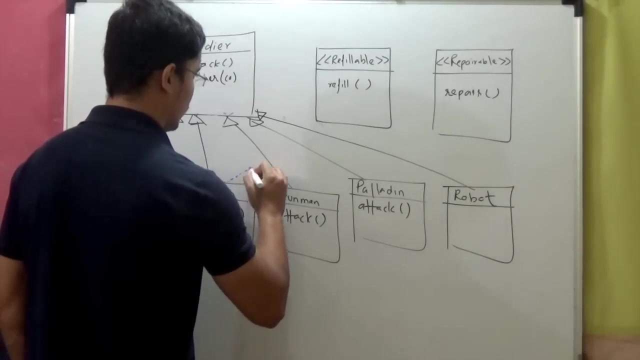 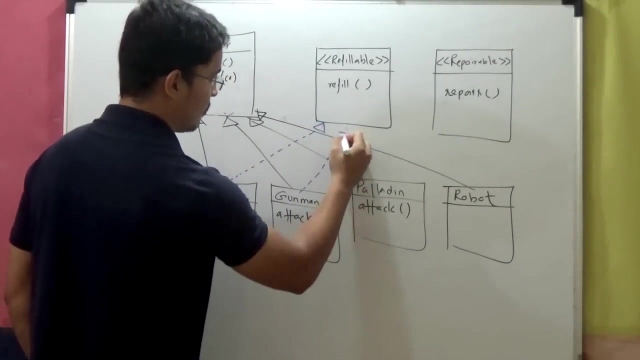 refill method. right, and repairable interface will have some repair method. some repair method right now, instead of i'll take out this behavior from here. and the classes which want the refillable behavior: archer: right, so archer needs refillable, so archer will implement this interface. gunman- gunman requires refill robot. robot also requires to. 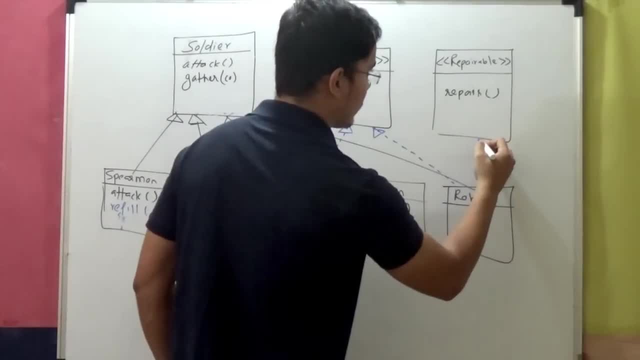 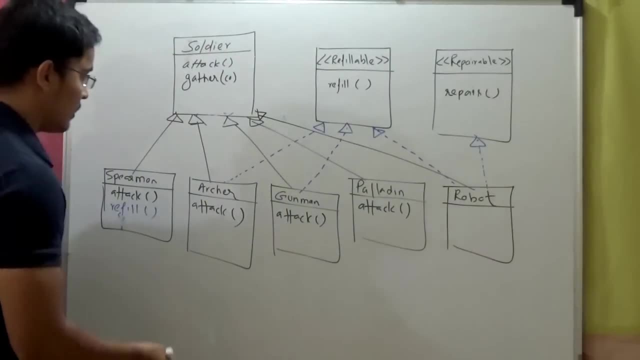 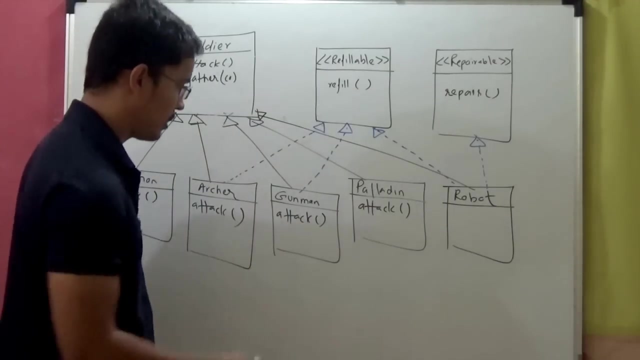 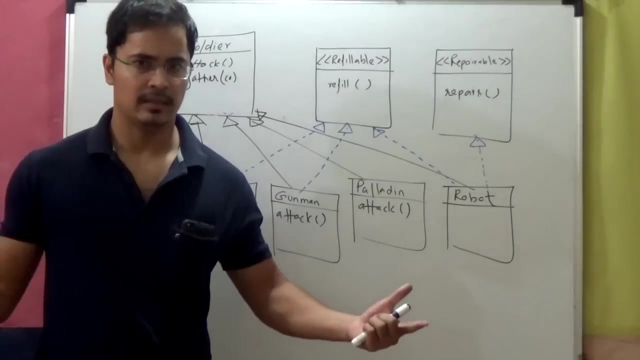 refill his weapons and robot also requires to be repaired in case it gets damaged while fighting. right now, we don't need to provide any implementation for refill in spearman and gunman- sorry, spearman and paladin, because they are not implementing this interface. sounds like a better design. 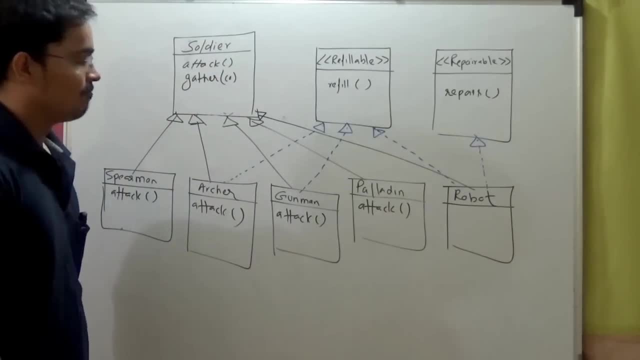 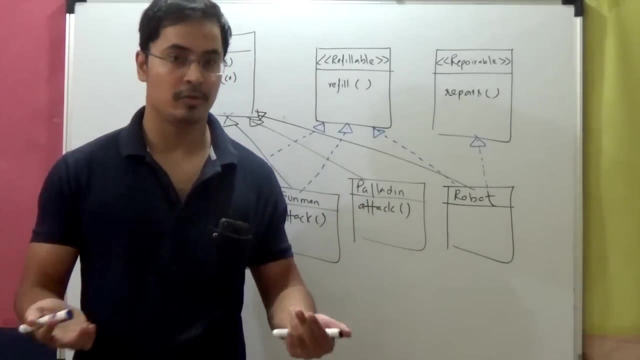 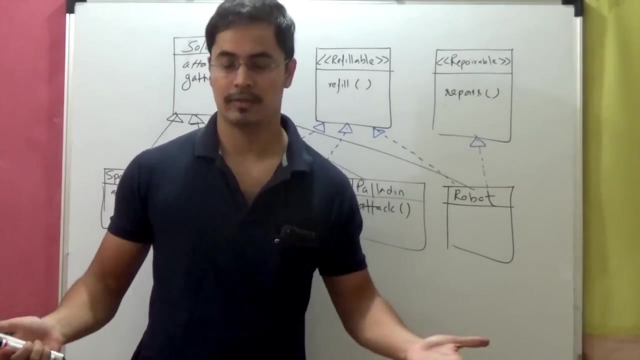 better way of solving that problem. right, but it doesn't end there. why software changes? i told you in in that video in solid principles: software changes, software changes changes. it keeps on changing. that's the only constant thing about software. requirements are going to change. so now they are saying that you know what this? 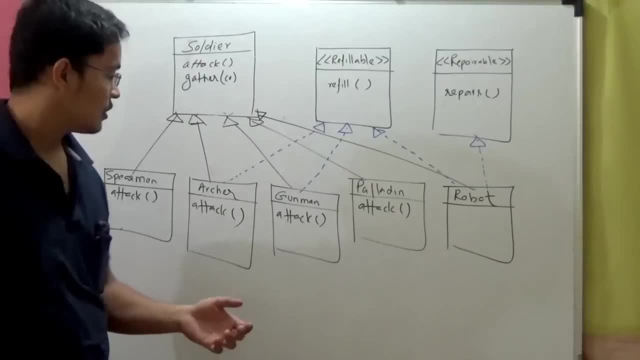 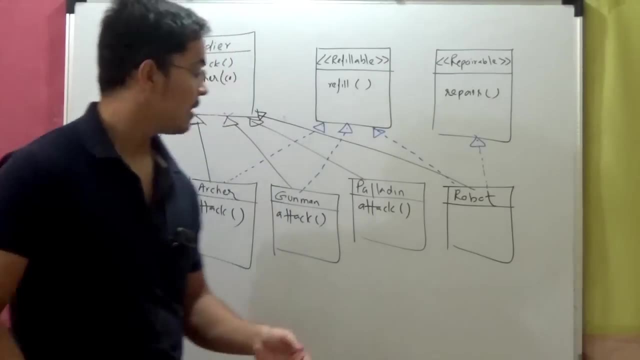 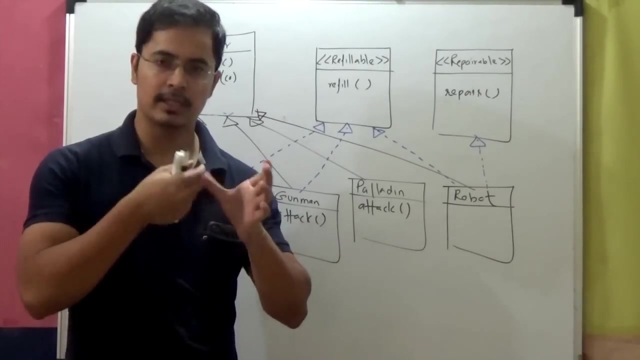 refill behavior. we want to customize it so archers will refill based on their number of arrows that they are carrying right and gunman they don't have, a gunman doesn't have. you can't show the bullets inside the. it's very tiny right on the screen. so they will refill based on some time, like after a certain period. 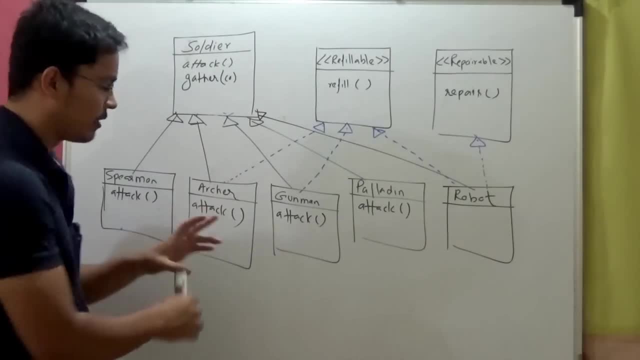 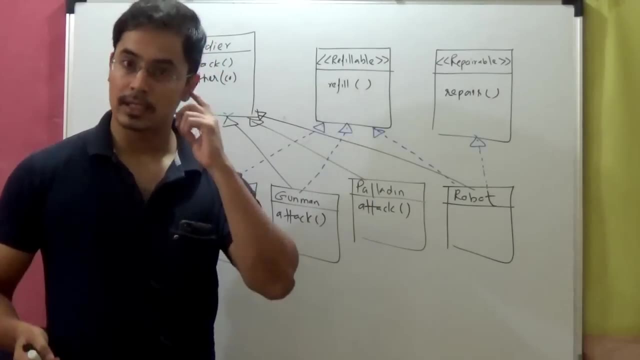 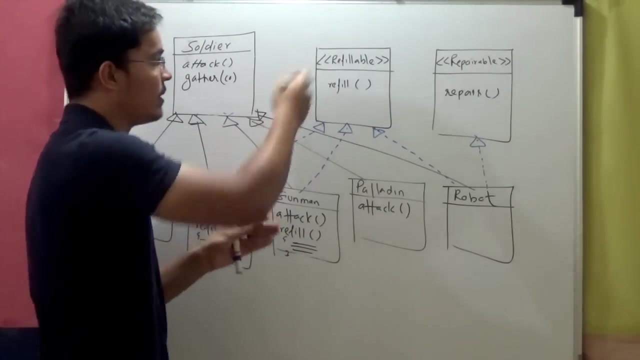 of time of attacking, they will have to refill. so for us it will be based on number of arrows for gunman, it will be based on time. so we want two different behaviors for this refill, so you have to change it. earlier it was similar right when they were implementing this refill. it was just time based. now there is a. 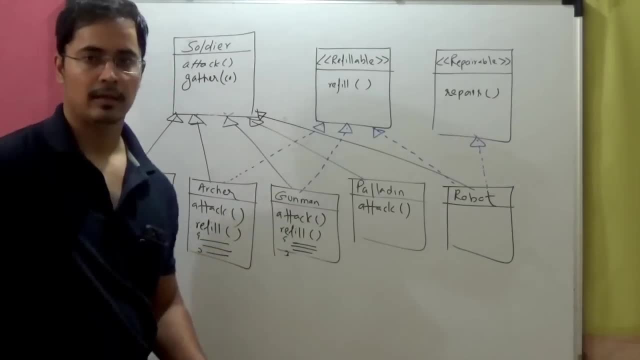 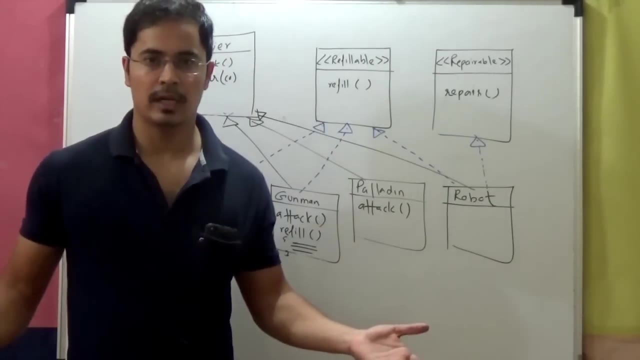 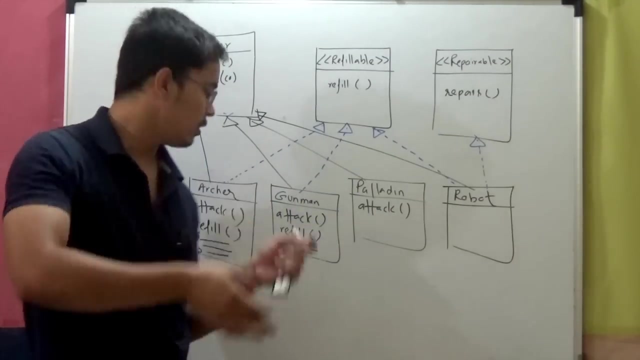 changing requirement so you'll have to make the code changes here. but these are just two examples. imagine there will be many more this kind of soldier which require the refill functionality. they will keep on adding new types of soldier. so because there's a changing requirement every time, you have to go in those respective specific. 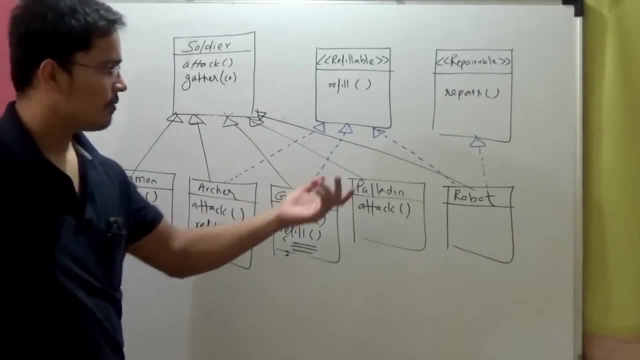 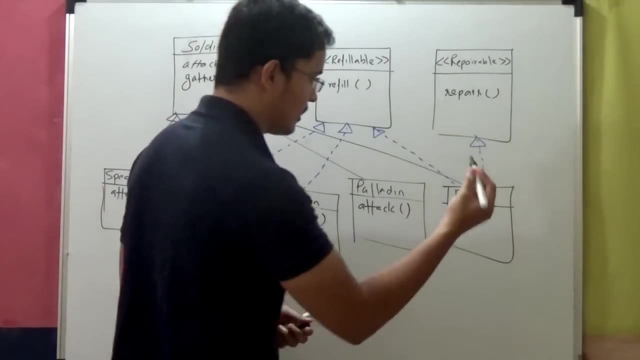 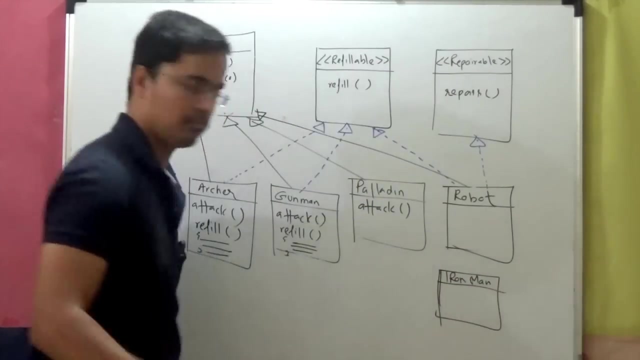 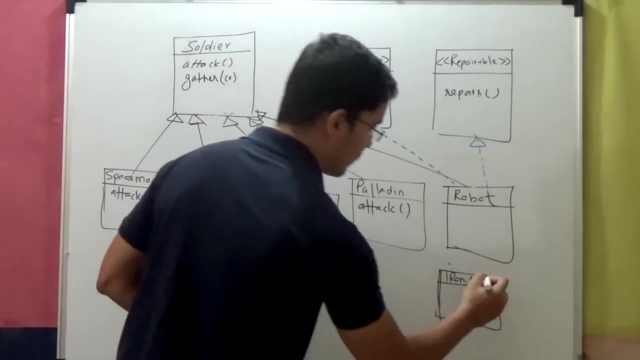 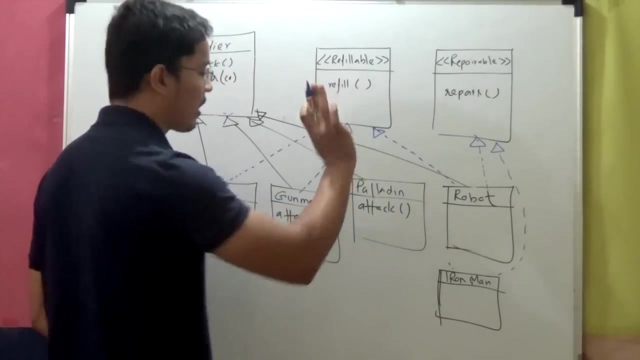 type and change the behavior again. they will say, now we want superhero kind of soldiers, so let's say they add another type, iron man. right, so there's a iron man type soldier, soldier, run soldier, arm carnage, and Sakurakaya has a Sort of Amid今日は iron man. 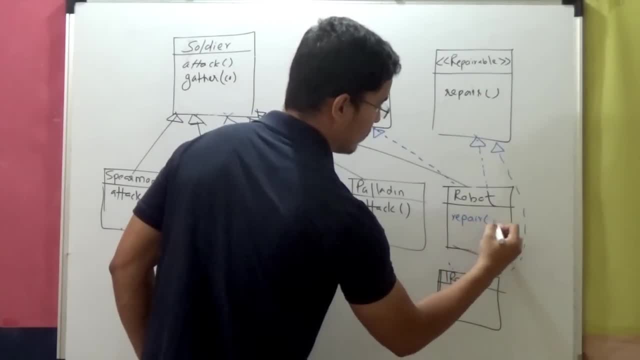 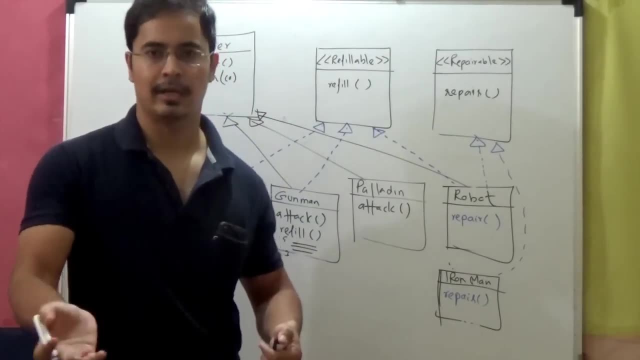 he will need to have a great, because Iron Man suit can get damaged. Ironman will probably, But then again they both implementing these repair right, robot and iron man. so this is Because they are similar, right? Iron Man also is a robot, basically Human inside a robot. 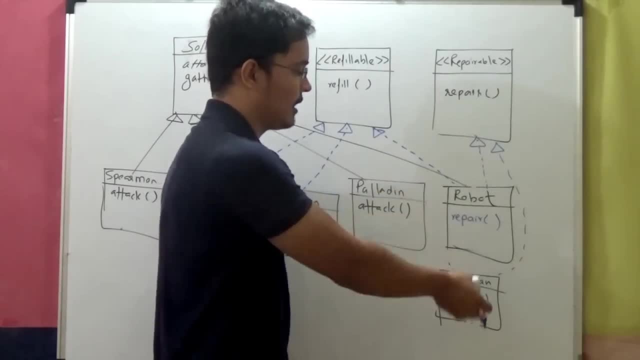 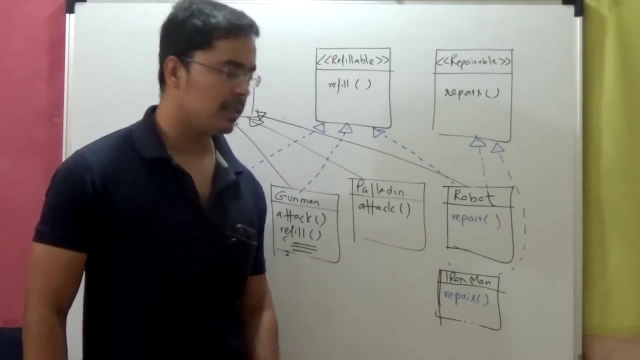 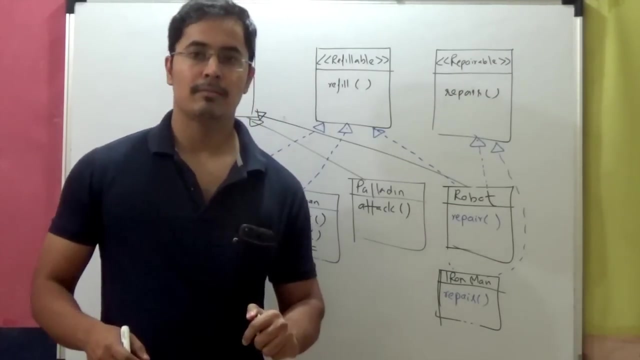 And robot is a robot. So they both have this repair functionality, But now change after some time And the team has decided that Iron Man's repair behavior will be different than robot's repair behavior. A robot will need a mechanic, a human, to repair itself. 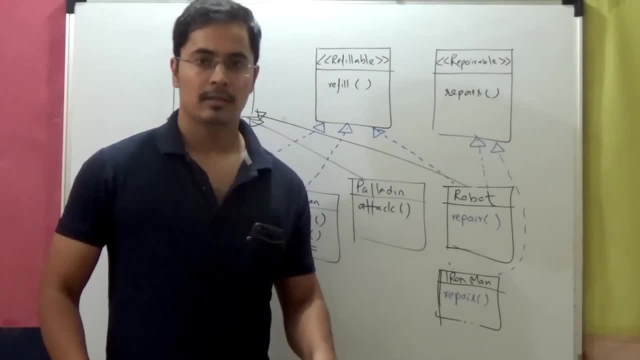 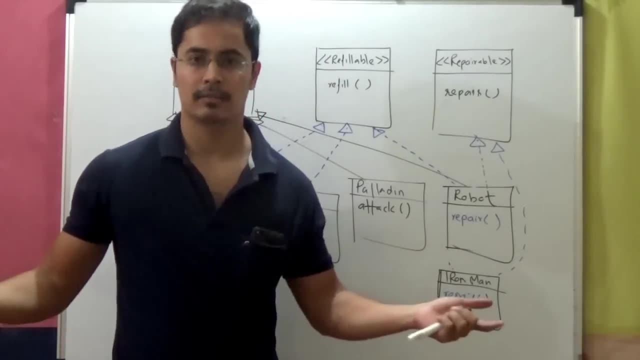 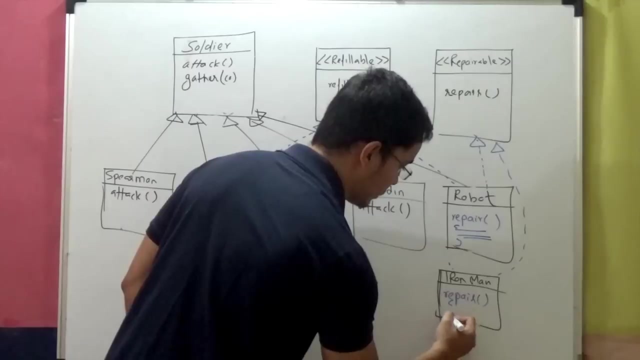 Because there is no human inside robot, But Iron Man. Mr Tony Stark will repair his own Iron Man suit or whatever that robot is. So you have to change. So here I'll have to write some another logic. Here I'll have to write some another logic. 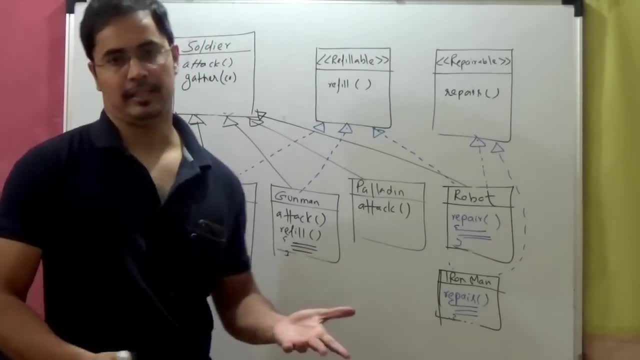 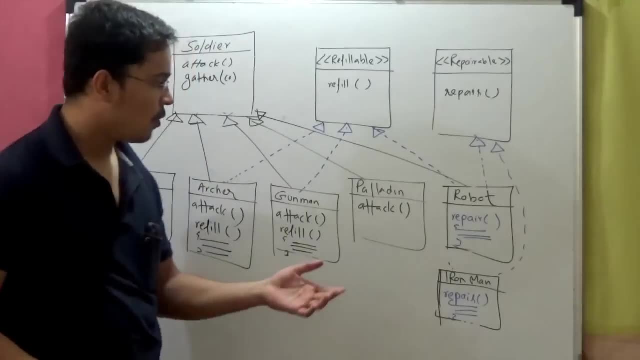 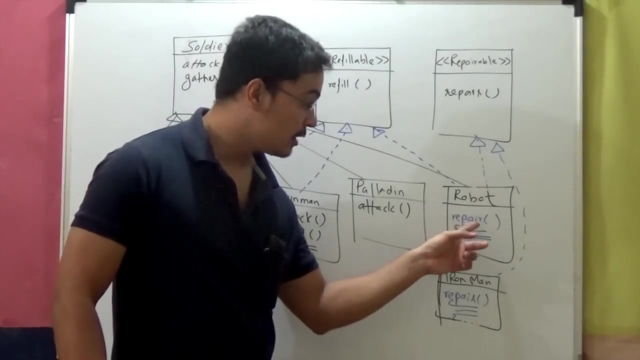 Again: Yeah, change A lot of changes, And we are only taking five examples of types of soldiers. But- And you are Because some, Because some behavior is changing, You are changing your types, You are disturbing the code of. 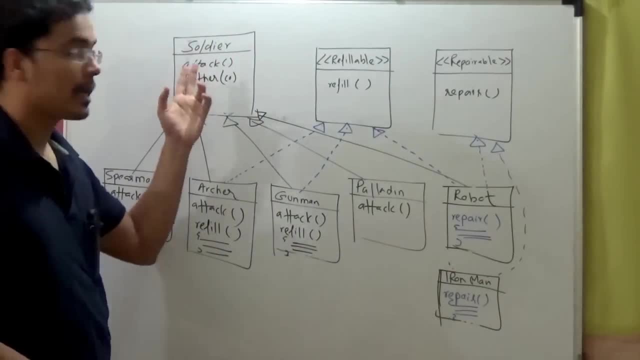 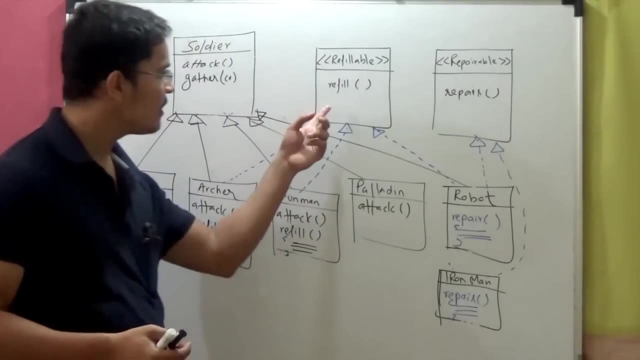 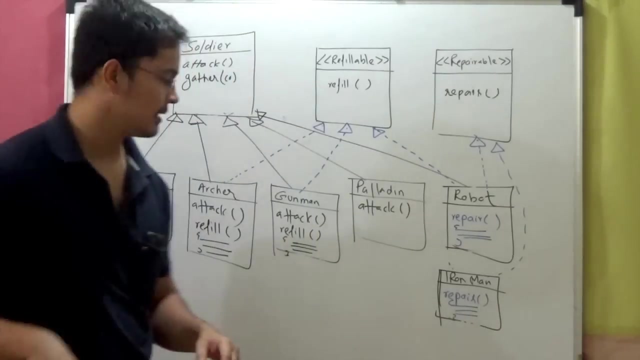 Robot will have some other functionality, Like gather, Like attack Like, Or Iron Man will have some other functionality. So this behaviors of refill and repair will keep on changing. Is it a good idea every time to go to specific classes and keep changing the code? 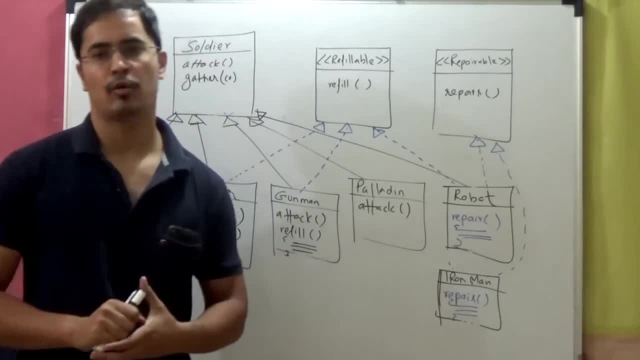 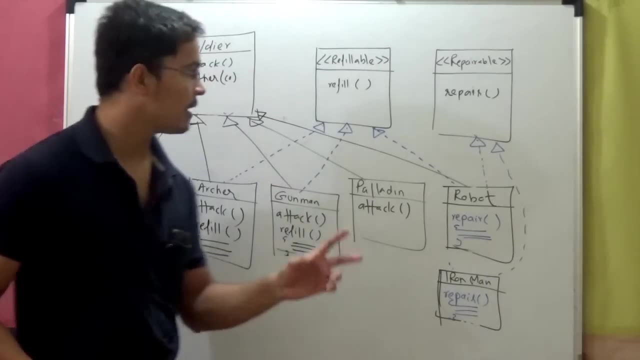 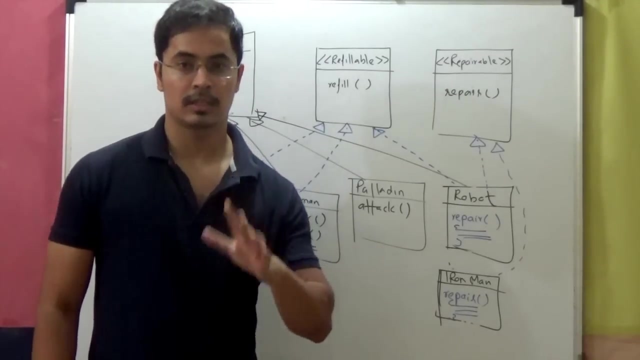 I don't think so. This is not a good design. It doesn't seem like a good design. So what now? How do we solve this dilemma of managing this change that is happening in these two behaviors of refill and repair? So the general rule of thumb, as I told you in the solid principle discussion: whatever is changing, take that out. 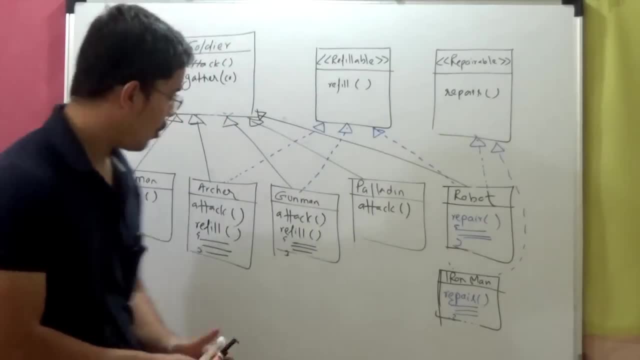 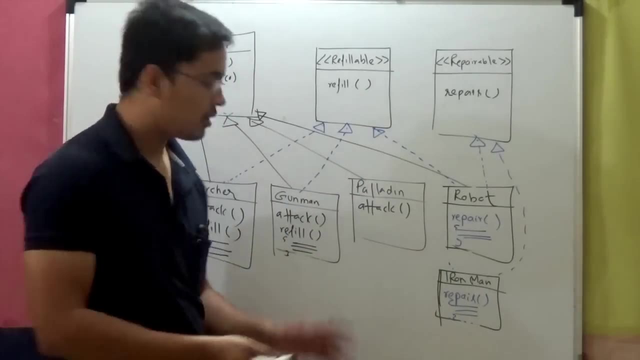 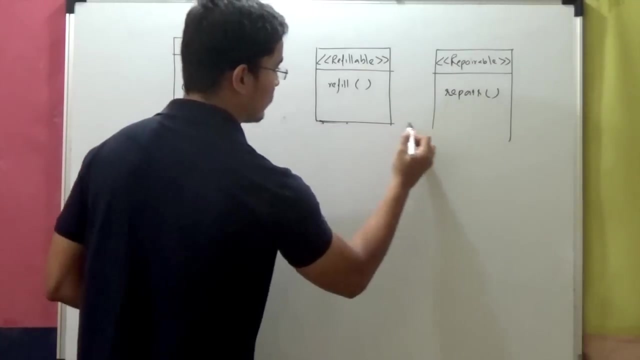 Separate it out from whatever which is not changing. So all these classes, what is changing? Repair and refill behavior, Right. So take it out. Don't keep it inside these classes, Take it out. So what we will do is that these are our interfaces. 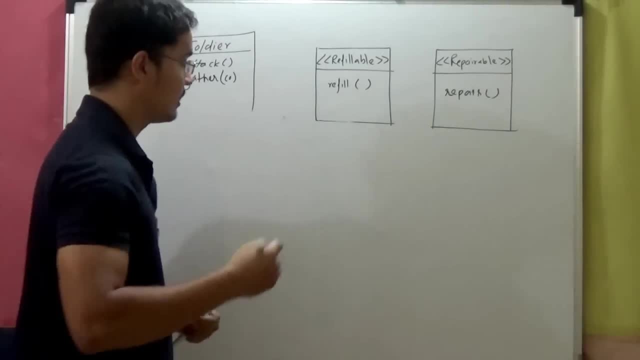 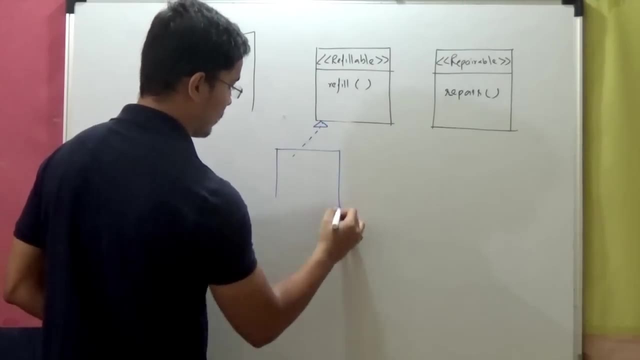 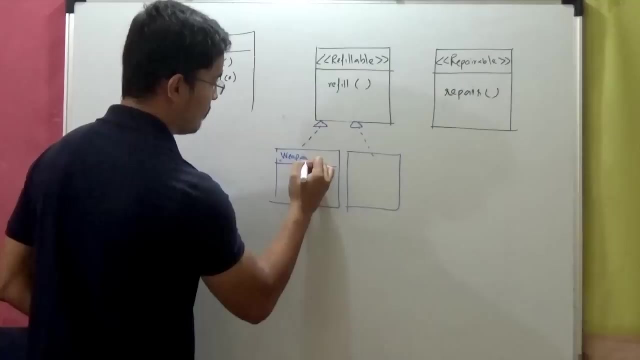 Right. So we will provide a concrete implementation, But we will encapsulate the behavior, So we will have a class Right Called as. So we know we have two kinds of refill behavior: Weapon based refill, And we have 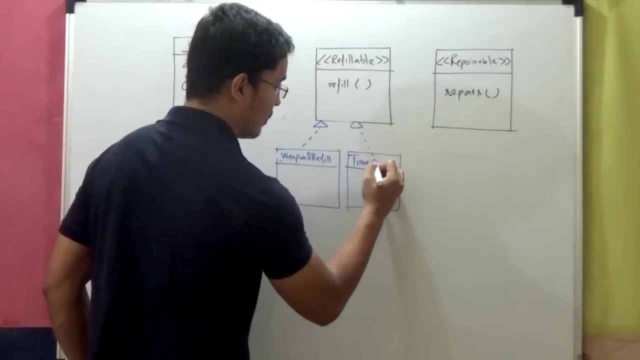 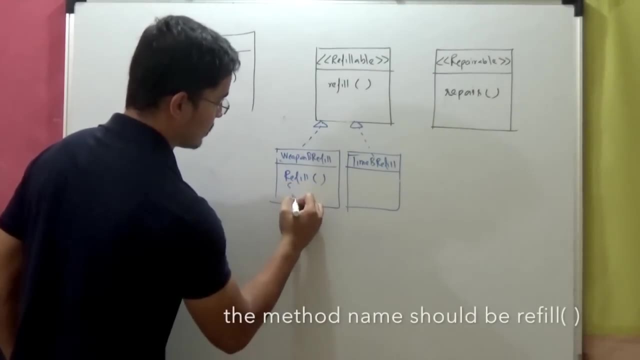 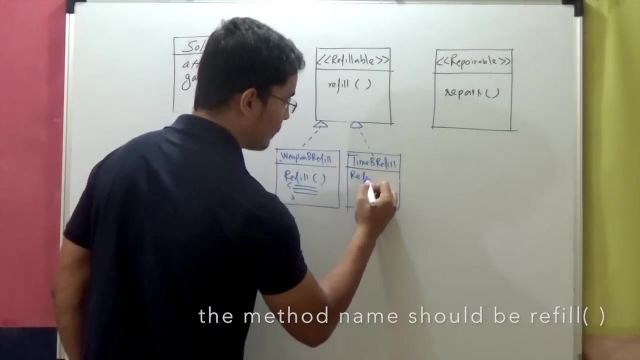 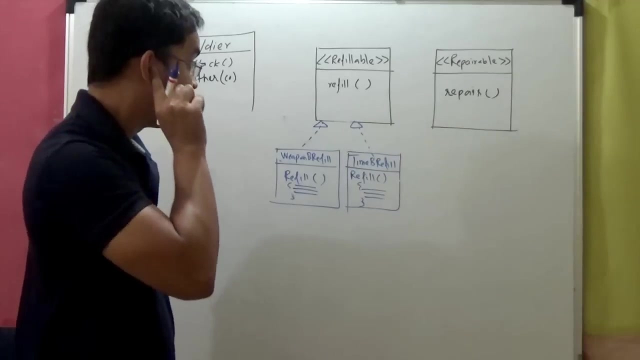 Another kind of refill, That is, time based refill. Time based refill- So here it will have certain weapon based refill, Like number of arrows, And time based refill will be based on a specific amount of time, Timestamp, Right. So in repair we have two types of behavior. 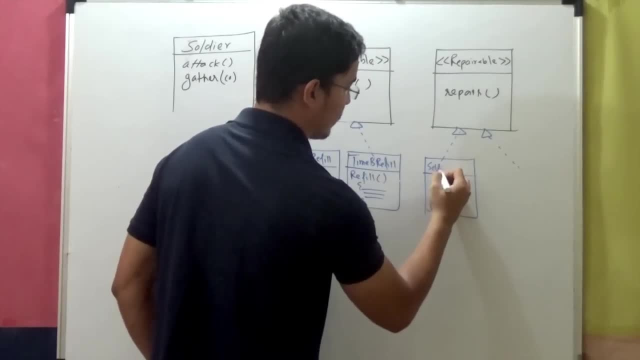 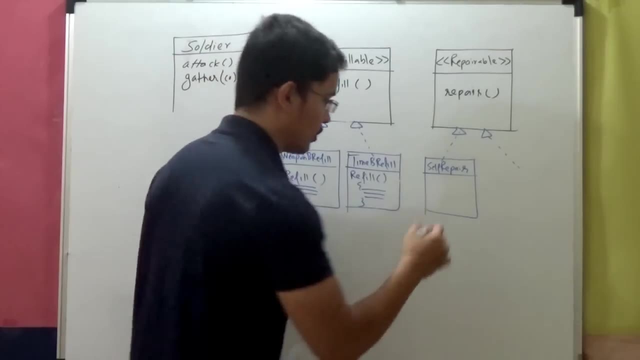 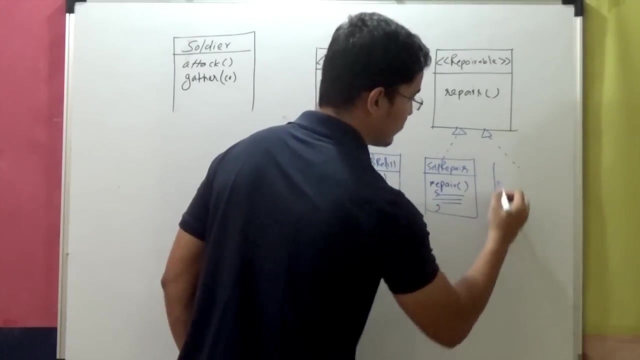 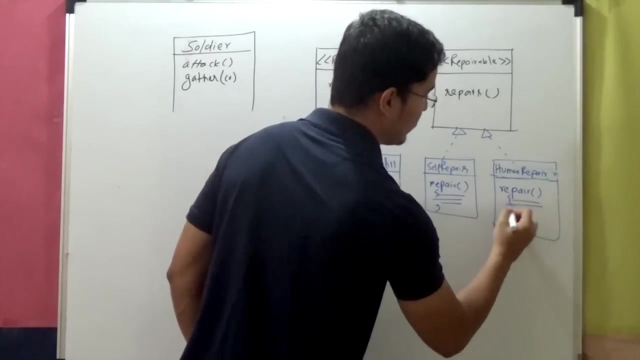 One is self-repair, That is, Mr Iron Man, Mr Tony Stark will repair his own robot because he is inside that robot while attacking. So that is one implementation of repair. And another is human repair, So this will require a citizen or a mechanic to go back to that. 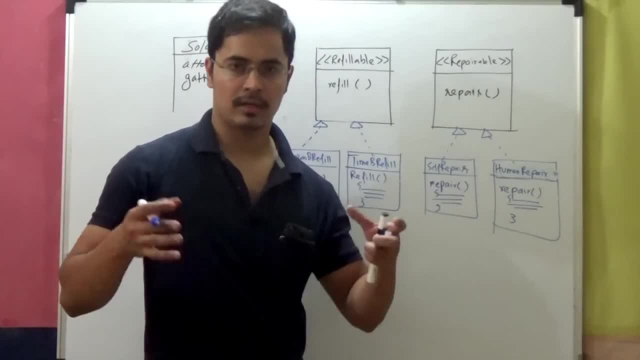 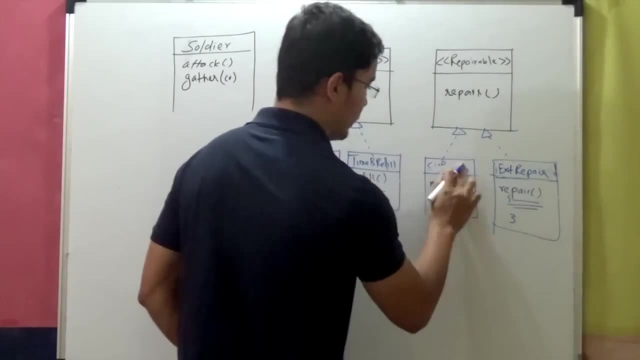 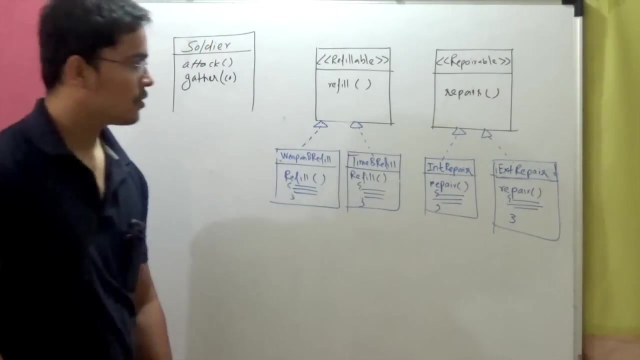 A mechanic will go to that particular robot And repair it And will repair it from outside. So this is: You can say external repair And we can say internal repair, Self-repair, Internal repair, Right? So what we have done is that. 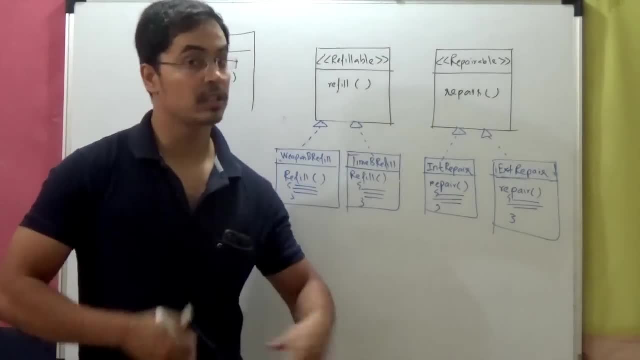 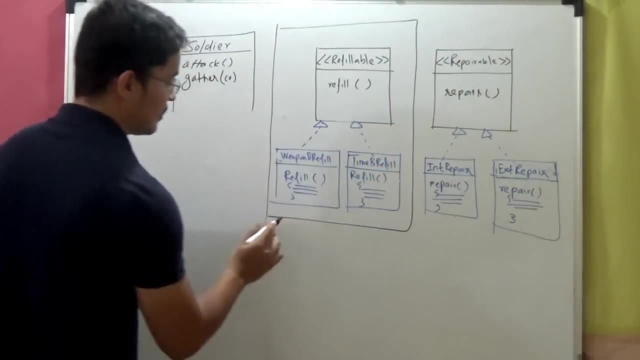 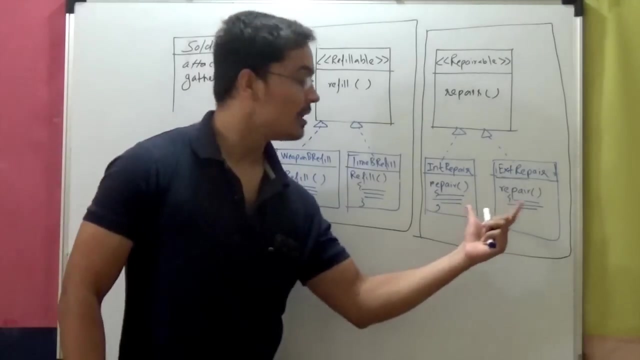 We have encapsulated the behaviors Because they were the ones who were changing. So now, If you draw this, So there is a family of algorithms. This is algorithm family For refill behavior. This is algorithm family For repair behavior. 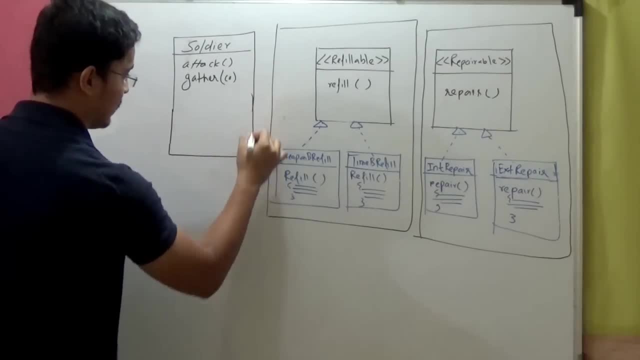 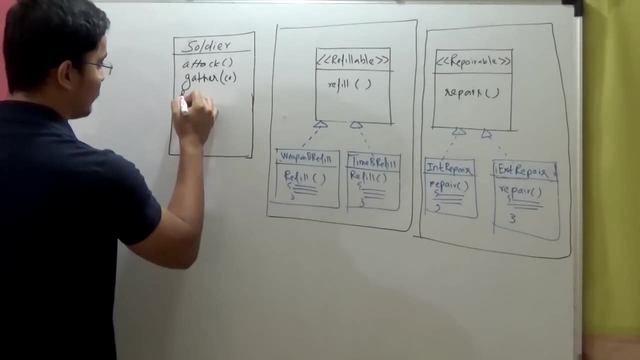 And now, One thing that we need to do here is that Here in the soldier base class, we will have a type of refillable composition. Refillable are, let's say, a composition and one instance of repairable. Now, while the child classes, objects are created. 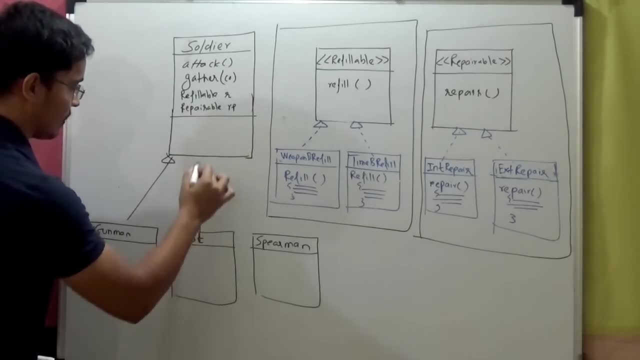 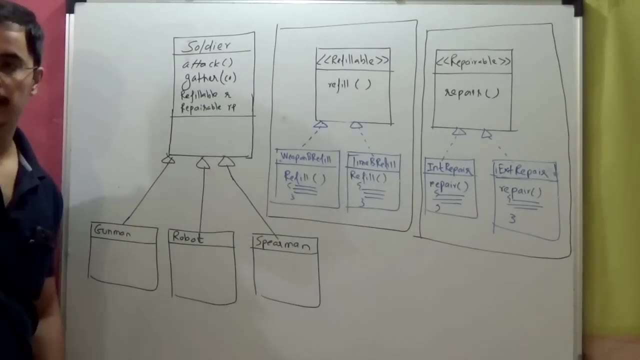 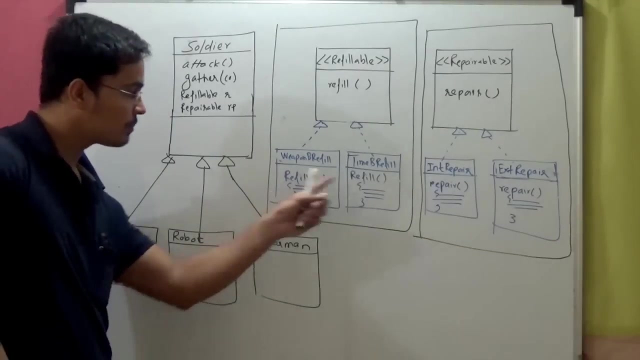 Obviously, these child classes are inheriting from this Right. While you create a child class object, you will have to create an instance of refillable Right. So now these child class objects can choose from these particular behaviors Right. We will also add one. 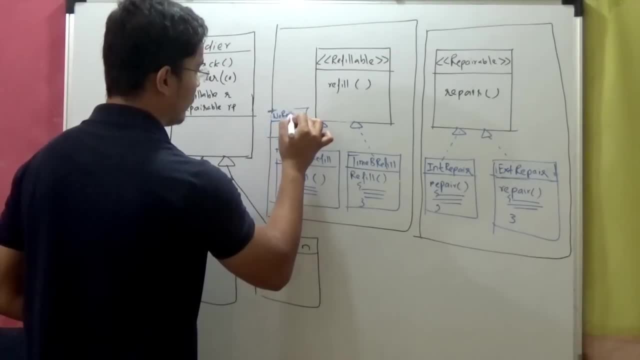 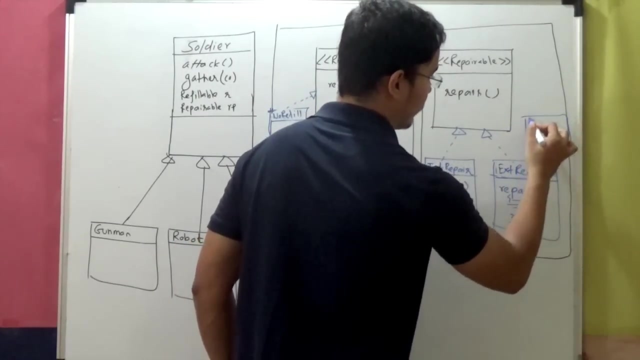 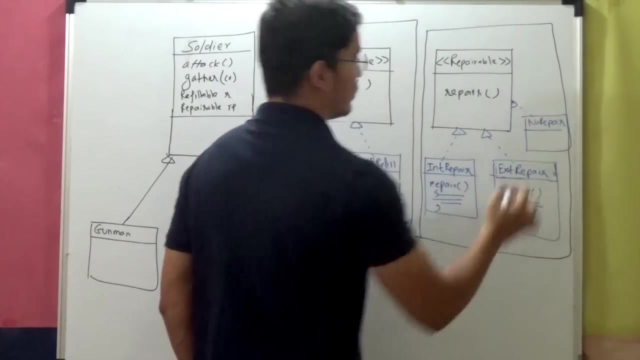 We will have one No refill behavior Right, So which will, Which will provide the blank implementation of refill, And we will have some No repair behavior Right Which will have some blank implementation of this repairable interface. So now Spearman. 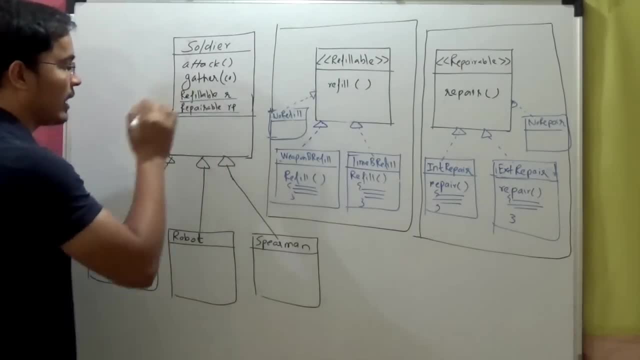 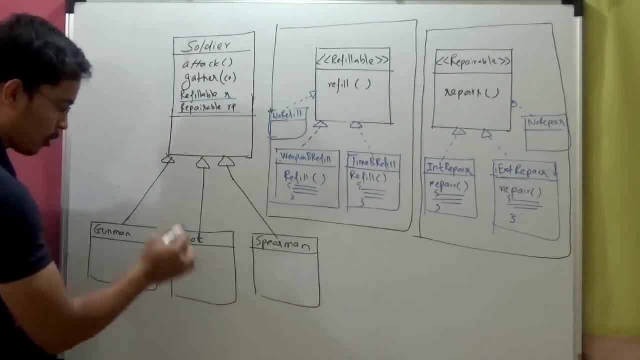 While you create the object of Spearman, For this contained refillable, It will provide the instance of No refill and no repair For robot. While creating the instance of robot, you will have to provide for this contained refillable So robot can use. 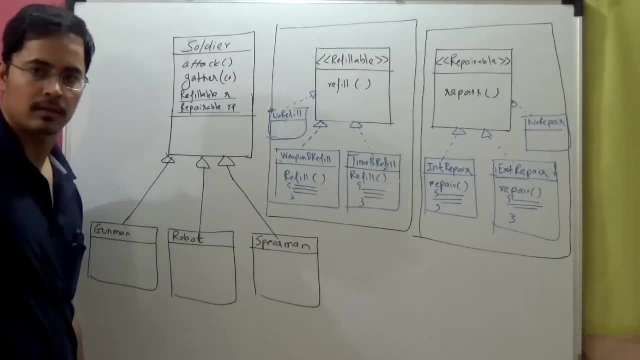 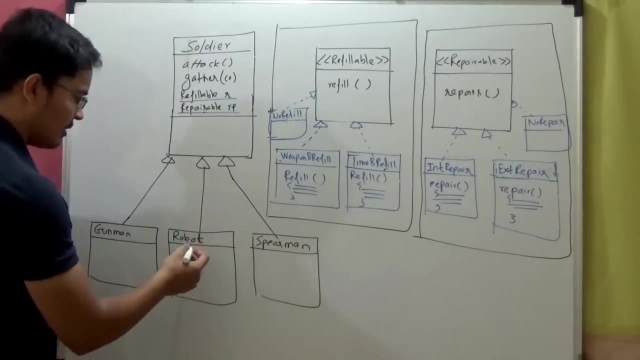 For refillable he can use time-based refill object And for repairable it can use external repair object. Right Tomorrow we want to change it, Or robot will also be internally repaired by itself. Then dynamically at runtime we can change. 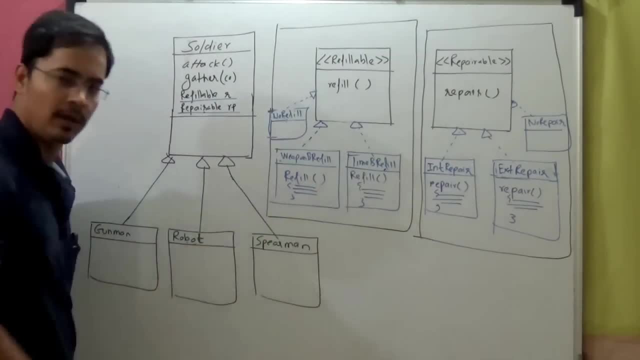 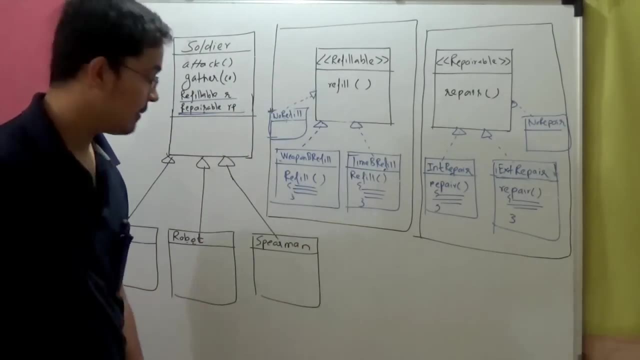 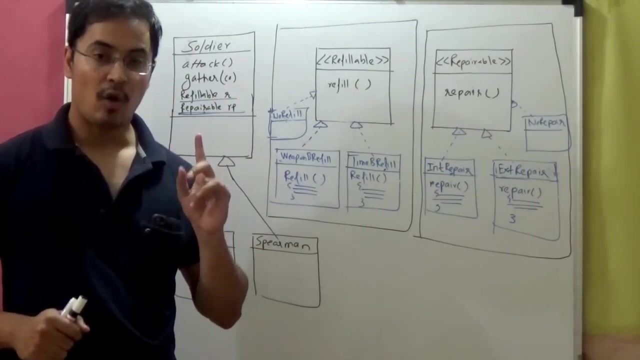 Robot will provide for refillable as time-based refill implementation, And robot will provide for repairable as internal repair. Right See now what is happening. One more design principle here is Always program to the super type, So you are using composition. 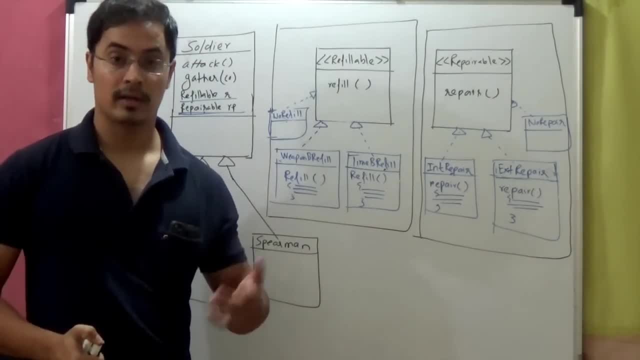 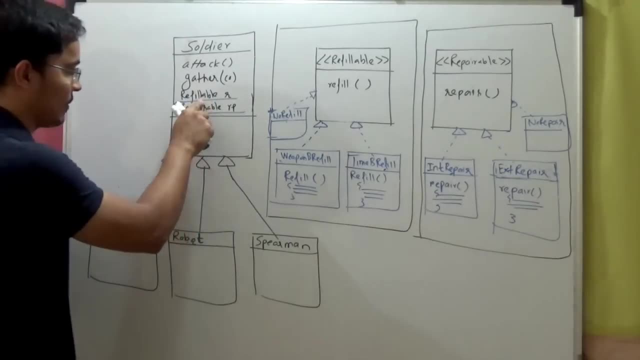 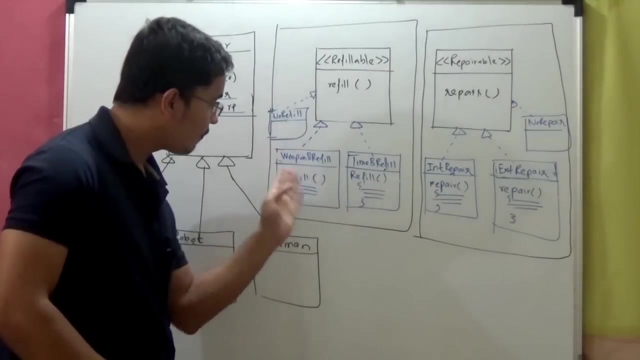 Sometimes composition is preferred over Over inheritance, Because composition is flexible, Much more flexible. Right, This is a super type, This is an interface. We need an instance of interface So at runtime you can choose from this family of algorithms. 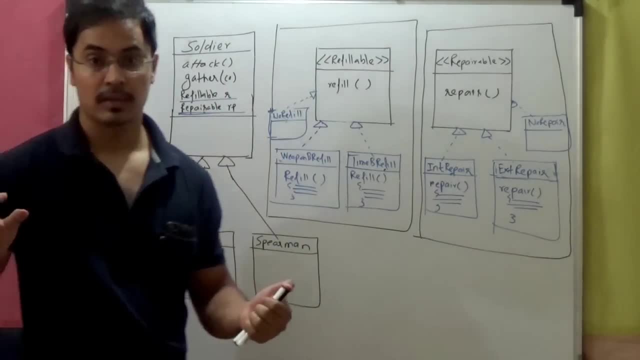 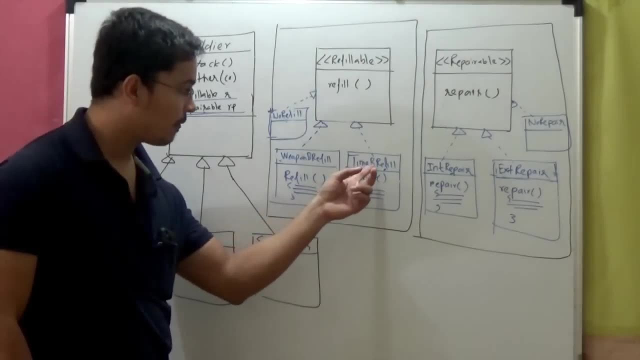 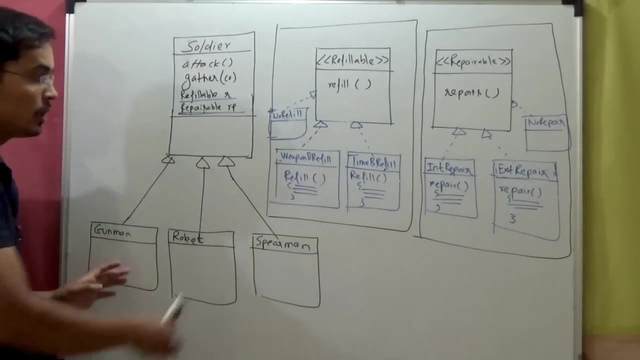 Right Robot instance depends on the business decision Depends on the functionality requirement. Robot can be created with the instance of time refill, Time-based refill Or weapon-based refill. Gunman can use any of this for this and any of this for this while they are getting created. 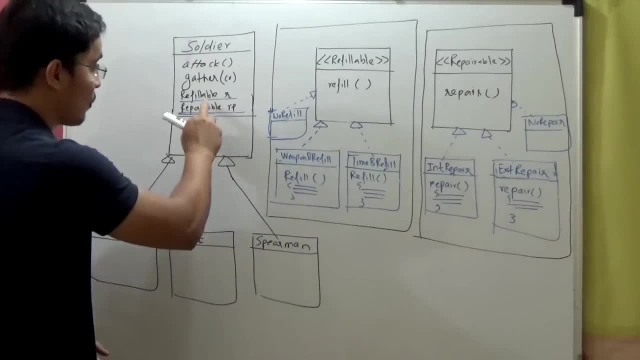 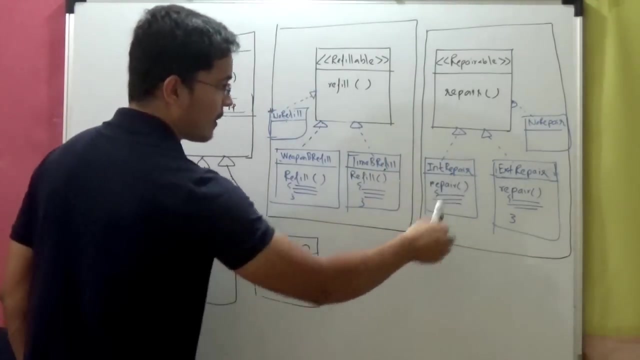 So you can change that runtime because you are programming to interface, You are programming to super type Right. This can be given instance of no refill, weapon-based refill, time-based refill. This can be given instance of internal repair, external repair or no repair.